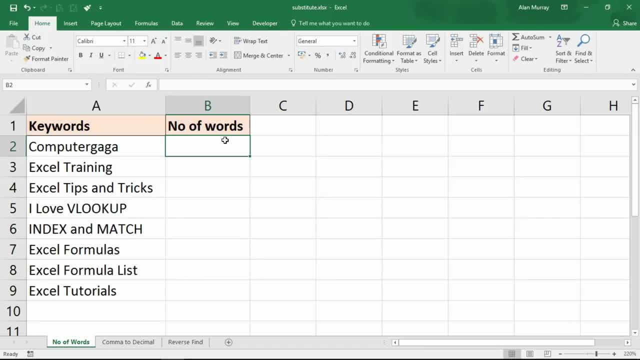 But we would like to find out how many words are in each cell. Now, technically, what we're actually going to do here to answer this scenario is find out how many spaces there are and add one on top, Because we know, if we can identify the number of spaces, the number of words will always be one more than that. 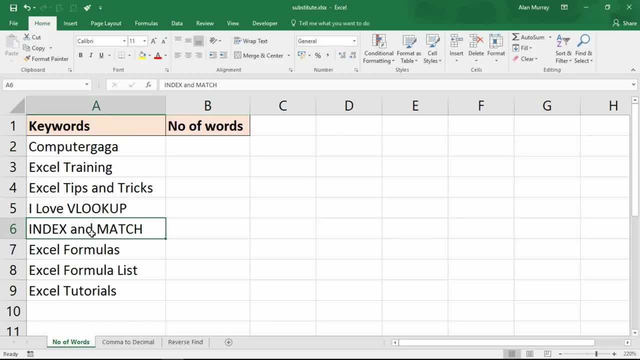 So index and match is three words and there's two spaces. ComputerGarGar is one word, There's no spaces, It's always one more. So that's how we're going to achieve this. So we're going to use a few different text functions. 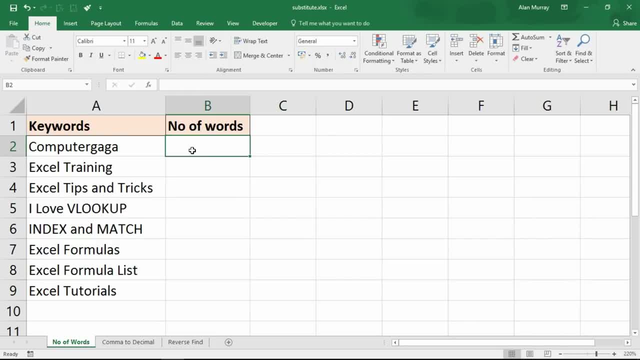 The substitute is the one that really gets the job done for us. First of all, we're going to use len. Now, this tells you how many characters there are in a cell. See, if I was to run the len function on that ComputerGarGar, it just tells me how many characters are in that cell or that word. 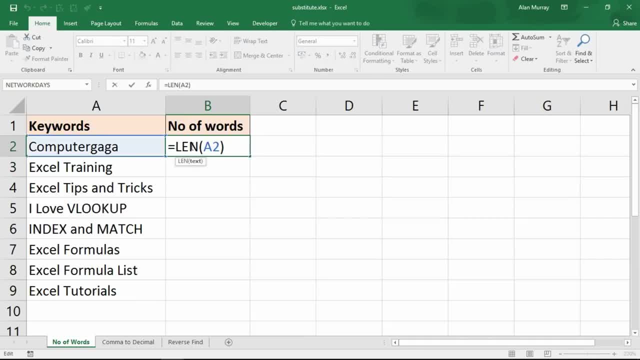 But what we're going to do is we're going to use the substitute function. So what I'm going to do is, if I can figure out how many characters there are in total, and I'm going to subtract from that how many characters there would be if I got rid of all the spaces. 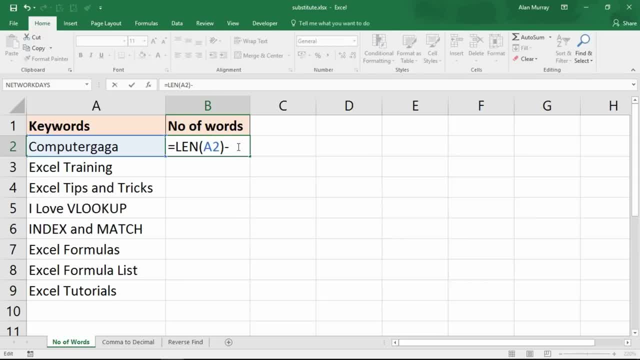 What's the difference between that? So if I was to put len in again, but this time substitute in there, Now, substitute just replaces existing text with new text, But there are so many reasons why that is useful. So in this example here I'm going to substitute any spaces that are in cell A2 with no space. 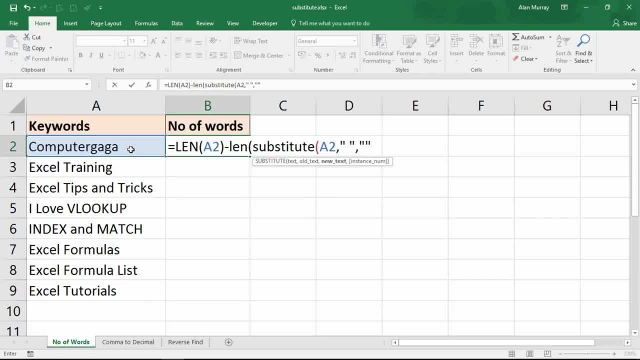 I'm going through this quite quickly here. This is not meant to be an in-depth tutorial on substitute. These are some quickfire reasons why we should love it as much as, hopefully, we do already, And I'm just building on your current love level. 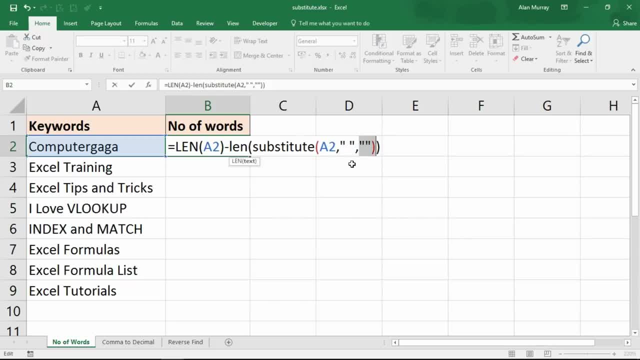 But here I'm replacing any spaces with nothing in the substitute function, Taking out all the spaces if there are any, counting how many cells. So if I press enter here there's none, There's no spaces. How many characters in total? 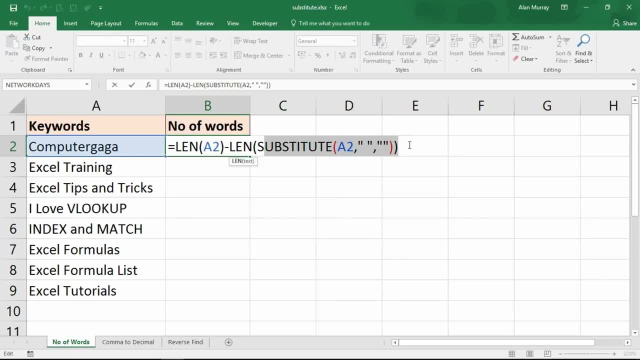 Take away the number of characters would be. if it took all the spaces out, There weren't any, so it makes no difference. If I copy this down, it tells me there's one space in there, three spaces here, two spaces here. 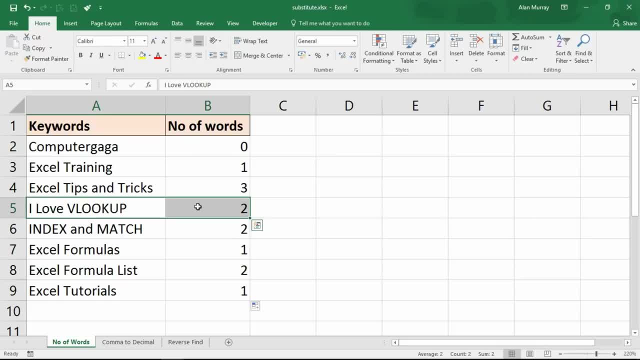 Now really, we're not trying to count the spaces, We're trying to count how many words there are. But we know there's always one word more than there may be spaces. So at the end of this formula, if we just put plus one, that will be how many words there are. 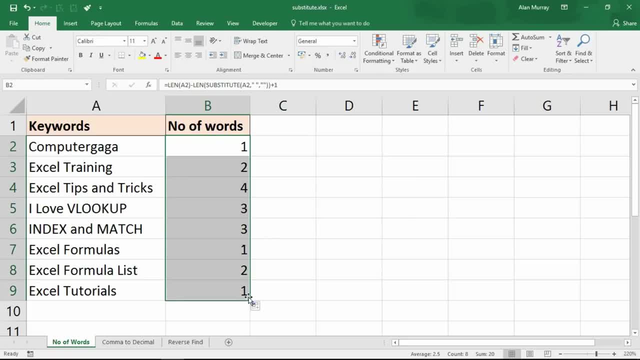 So there's one word now in the computer gaga, But there's two for Excel formulas and four for Excel tips and tricks. Now in this example, this is working on the theory that there are no erroneous spaces, leading and trailing spaces. 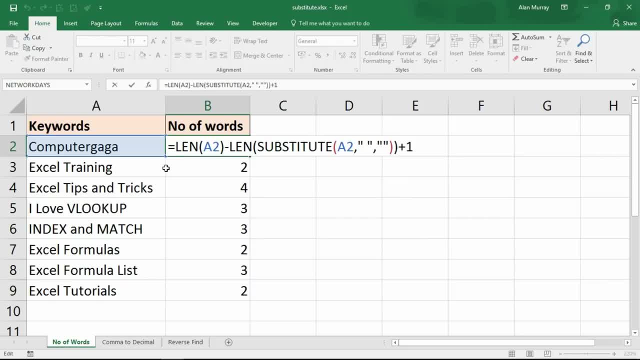 which is a common situation when people tie up and paste data into a cell. Now, if we wanted to protect ourself against that possible situation, we could use the trim function as well around the occurrences of A2.. It involves to trim that cell. 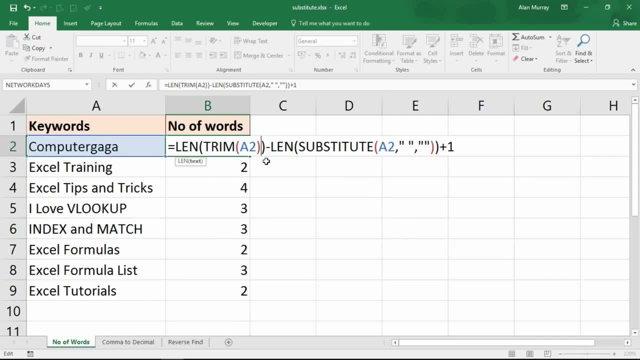 That would remove any excess spaces between the words or on the end of the string. And then I can kind of repeat that I might just copy that one and just paste it in instead of this A2 bit here. So I have a trimmed version of that A2.. 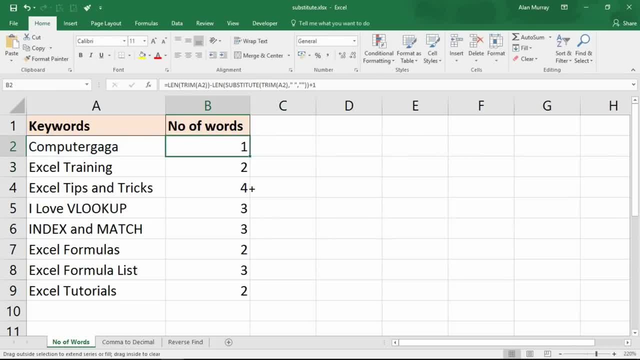 And when I press Enter here and copy it down, it will make no difference, But because that trim is there. should there be excess spaces on the end of a cell, like A3 here, it makes no difference to the result, Because that trim function is going to destroy those excess spaces. 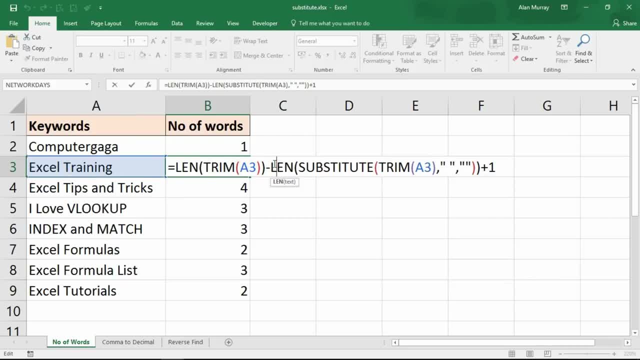 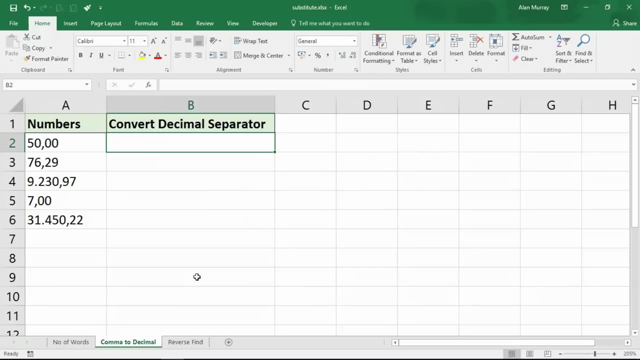 keep the one in the middle. that's a normal space, and then the formula does its thing. So that is example number one of the substitute function. Okay, example number two here, where we will use the substitute function to convert to the decimal separator. 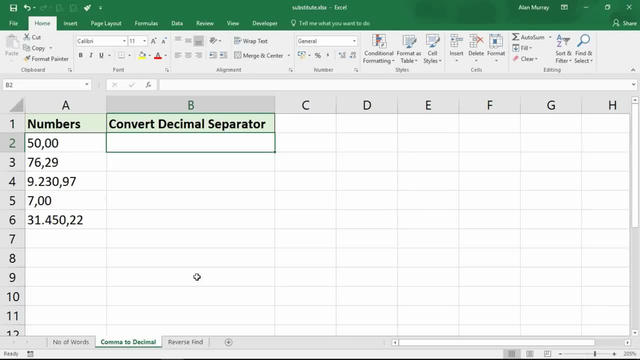 So I'm using the example here of a question that has come up quite a bit on my training over the years, where, when we're dealing with values from European systems, they may conflict with what we use here in the UK or in other countries as well. 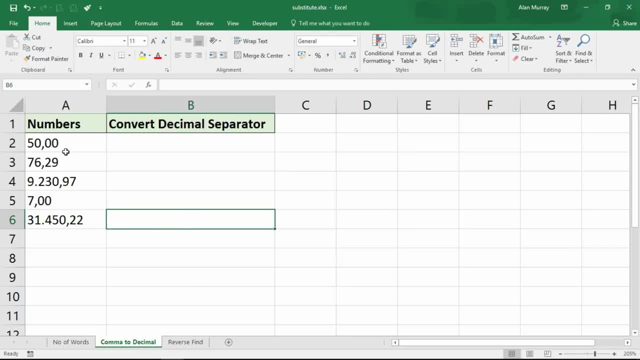 Whereas in most of Europe they will use a different decimal separator to the UK. Whereas we would use a full stop, they would use a comma. So, imagining that these values on screen have come from a database or system based in parts of Europe, 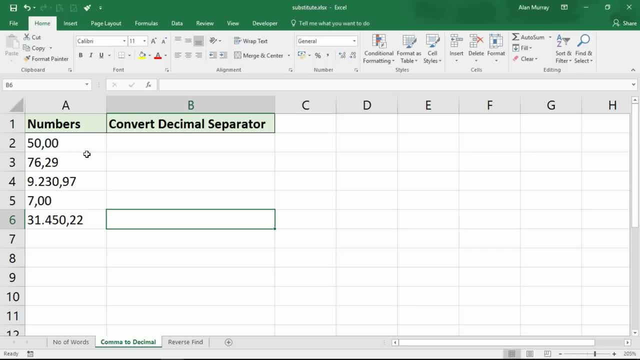 and it's coming to my Excel here and it looks lovely, but it's absolutely useless to me because my local settings are not recognising and understanding what they are. Good news: substitute function is going to sort those out for us, So we're going to use two substitute functions this time. 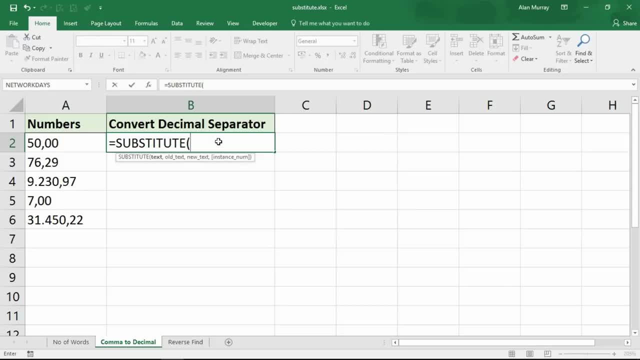 One is not enough this time, And what the first one is going to do is get rid of those full stops. The full stops are being used here as a thousand separator, whereas typically in the UK we'd use a comma for that. But we wouldn't need to type that in anyway. 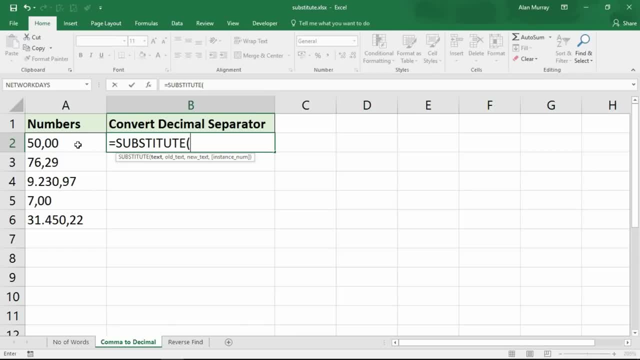 We'll do that with formatting, So I'm getting rid of those. Let's select the first number put in a comma, Let's put in a full stop And replace that with nothing. I'm taking out those full stops. Now we're going to use another substitute function. 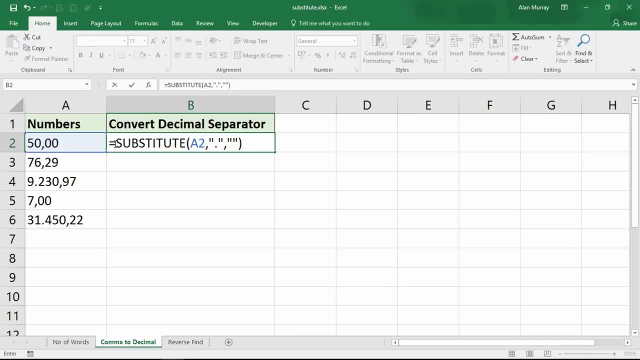 to convert the commas in those cells to a full stop, which is what I would use as the decimal separator here in the UK. So just outside the one I've got, if I start another substitute function- and I'm going to use the answer I've got there as the 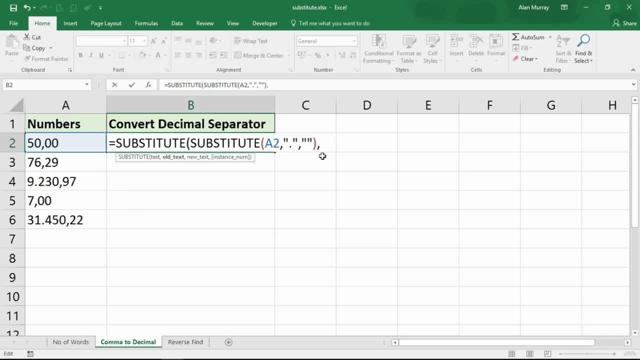 text value. Put a comma after it. The old text will be a comma And then the new text will be a full stop Close bracket. So that might look a little bit crazy with the commas there, This one being an argument separator. 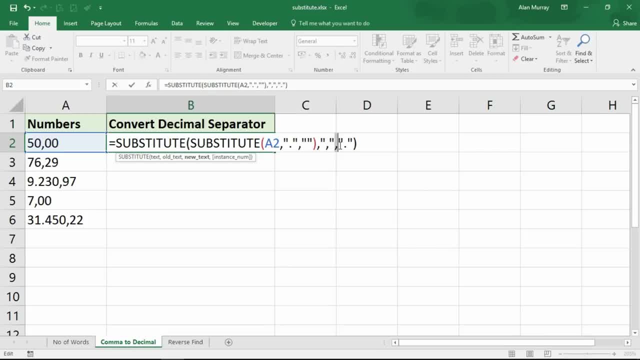 That's the one we're replacing. Another argument: separator: there There's a full stop. Replace the comma. We have a full stop That comma there. sorry, Sorted, That is what we want. The last thing really is to wrap the value function around that. 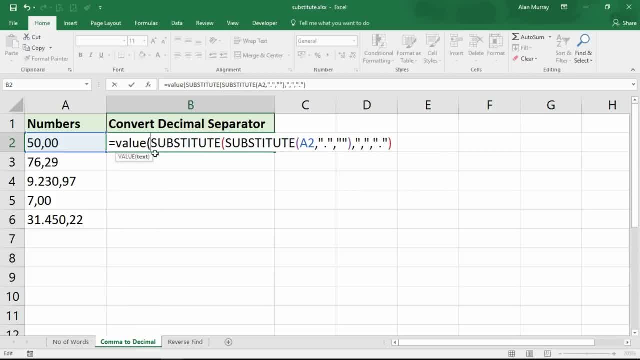 Because substitute is a text function. although it will change the separators like I want, it will remain as a text value Stored as text. So the value function is there to convert it to something numeric. So if I now press enter and copy this down, 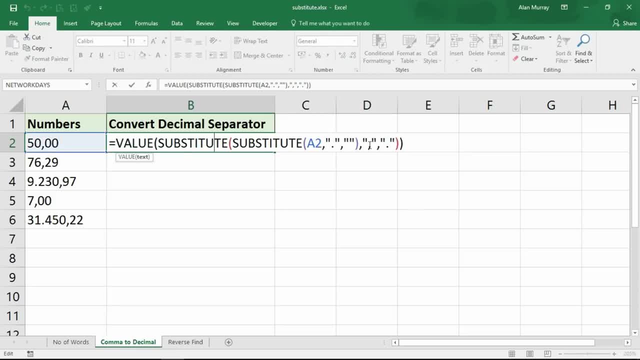 No full stop there necessary, Despite the formula saying: replace a comma with a full stop. And there is a comma, But it hasn't replaced it Because it knows that's a decimal separator and it doesn't need to. But if I copy this down: 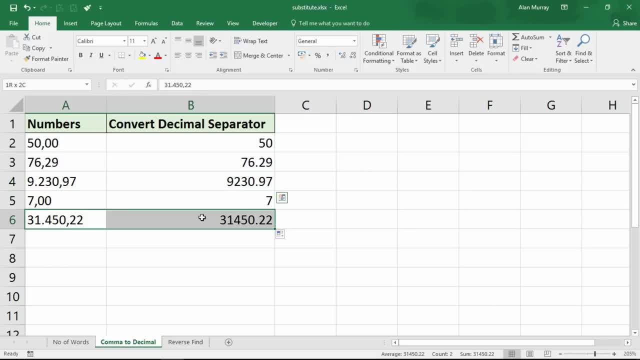 It does with value 3 and value 5. Because now it is necessary to do so, I can now format them in the appropriate currency, Whether that be US dollars or whether it be the British sterling. So if I was to choose my local currency, 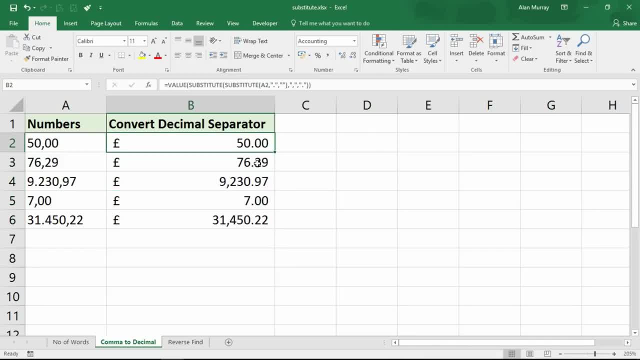 That looks horrible. That would have wired that column, doesn't it? But here we have it. We have the correct value, most importantly, Ignoring the currency settings, So that I can add them and chart them And anything I may need to do. 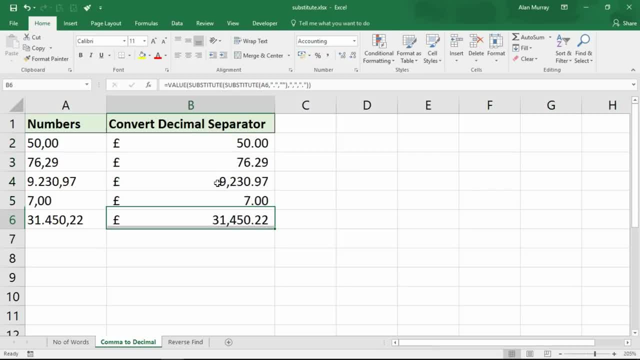 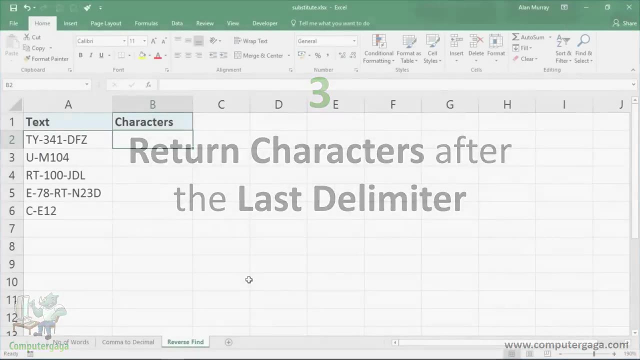 Whereas previously they were useless to me, But now they also look the part as well, Which is good too. Got the thousand separator in now, Because I've formatted it in the appropriate accounting format. Okay, Example number 3.. And the biggest formula yet. 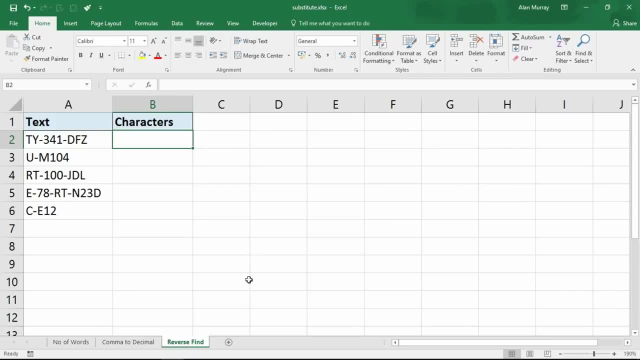 Where we use the substitute function To return all the characters After the final instance of the delimiter character. So there are different techniques in Excel, To you know: split text by a delimiter character, Or return characters before it, etc. But now we've been quite specific with the final instance of one. 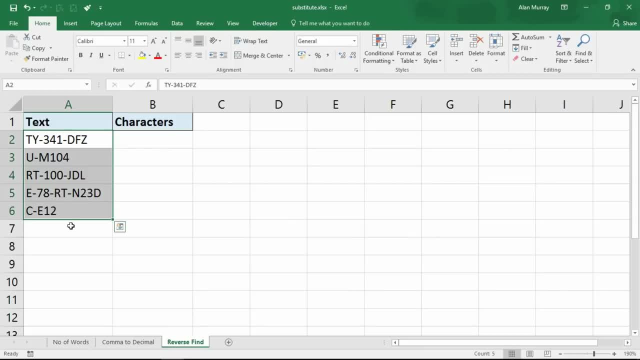 So, looking at these text examples, We have kind of two hyphens in the first one And the characters after. the last one will be D, F, Z. Got one hyphen in the second one, The characters after. it is four characters. 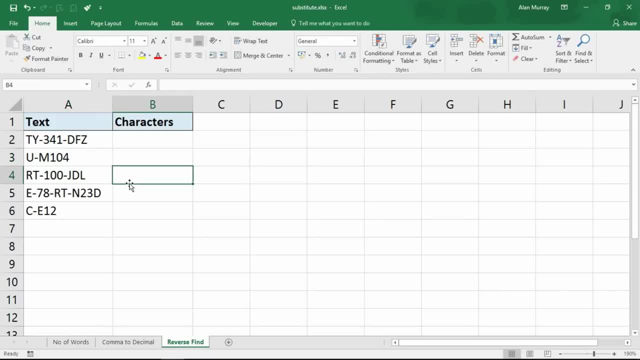 M104.. So they're quite irregular, The values in that column. All I know is that after the final instance of a hyphen I want the stuff after it. So this is going to take a bit more work, But once again, 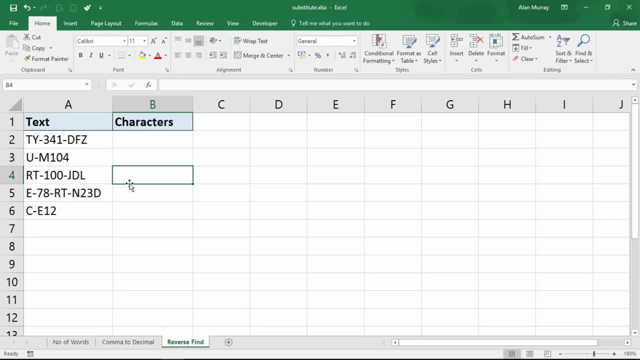 In the substitute function. We'll be up for it. So the first thing we need to do Is we need to find out how many hyphens Are in each of those cells, And the good news here Is that we have already done that. 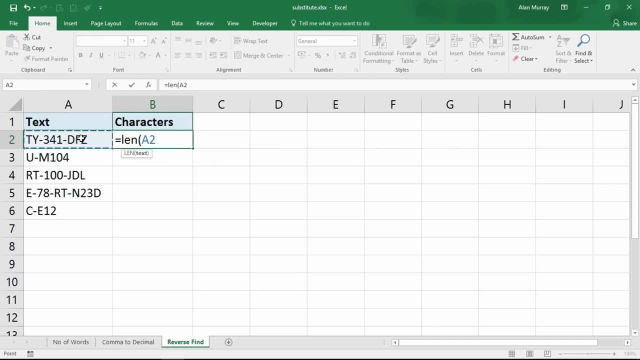 In this video. We have, in the first example, Found out how many words in the cell, And we did that by finding how many spaces plus one. Very well, basically the same Technique. here I'm going to do the len function To find how many characters in that cell. 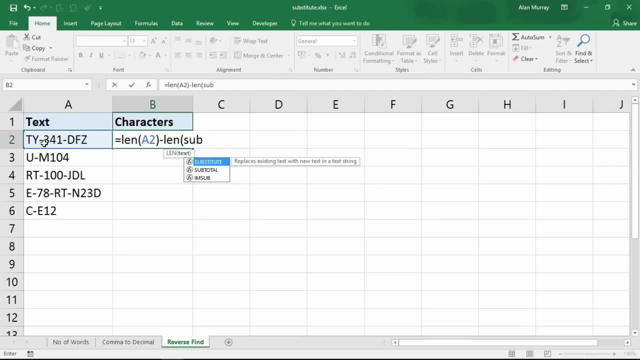 And subtract a version of that cell Without the hyphens. That will tell me how many hyphens There are. So substitute A2.. Oops, Comma The hyphen. Replace with nothing. Close. substitute close len. 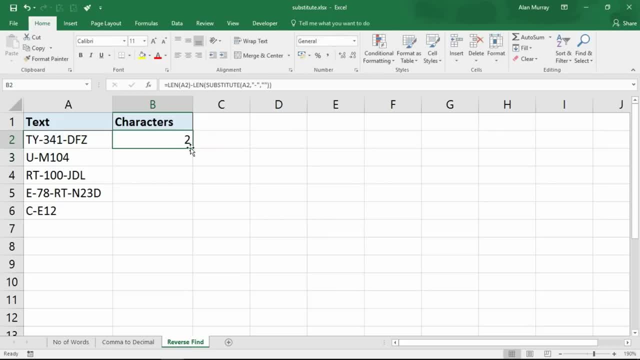 So if I press enter, It tells me there's two hyphens there, One hyphen here, Two there, Three there, One there, As we can see Now. Please don't be misled into thinking It has to be a hyphen. 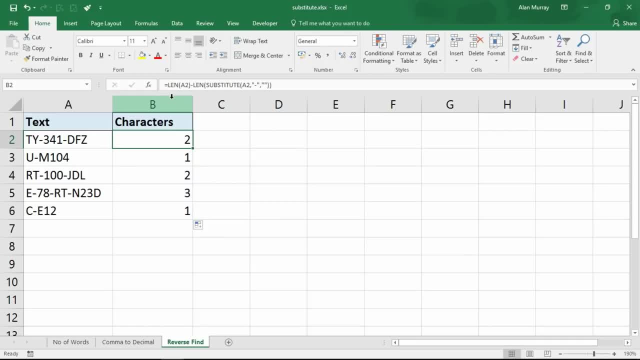 This can be any decimal, Yes, Or any delimiter character. A real common example of this Would actually be a slash. You know So when we're dealing with file names And URLs And trying to return Information after the final slash. 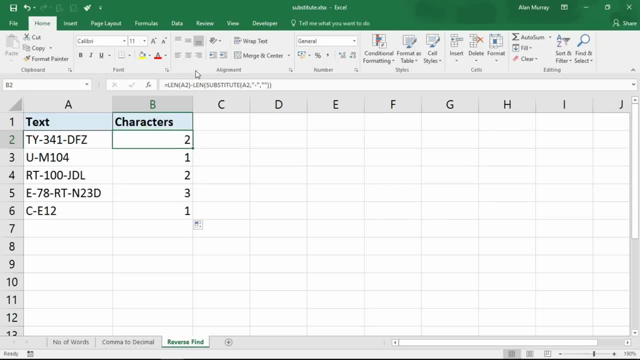 Or the third slash Or something like that, To get a certain folder Or file out of a directory Or web address. It's a very typical example Of this kind of thing. Okay, Now, Moving on to the next part. 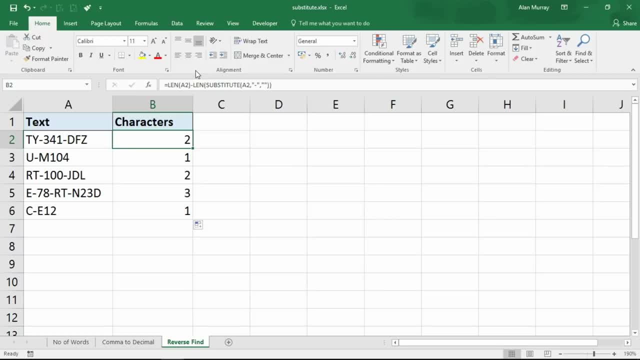 Of this formula, Because we're certainly Not done yet. So now we know how many Hyphens there are. We want to put a flag down In the last one So that we have a unique Way of identifying it. 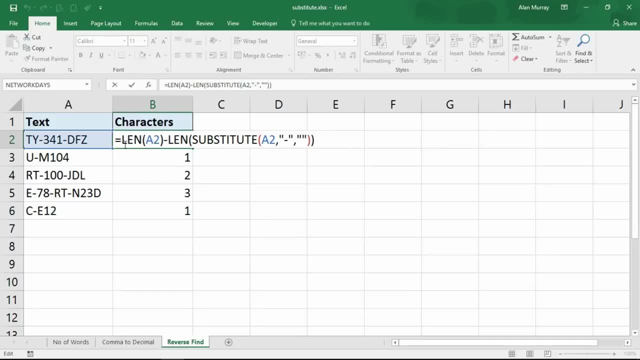 So in this formula At the start of it, Here comes another Substitute function, And this substitute function- Whoops. This substitute function Substitute Is going to be used To in A2.. Replace any occurrences Of a hyphen. 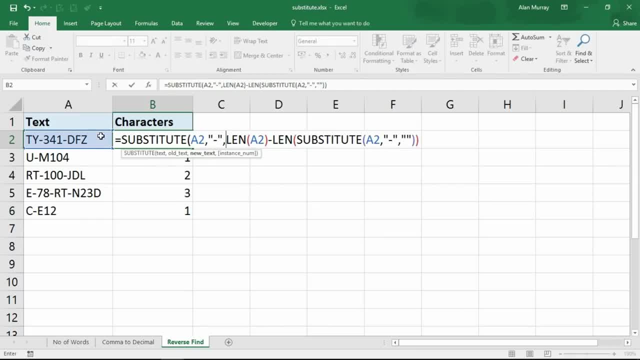 With Some kind of Of a marker. So I'm going to use a asterisk here, But this could literally be Any character, But I want something unique. So I'm picking an asterisk, Because there aren't any of those. 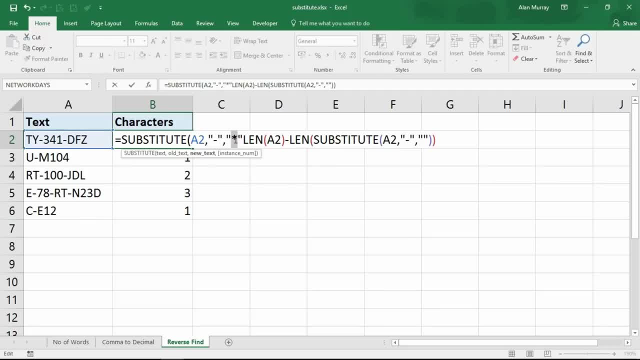 In these text values, But some kind of unique character Could have been anything, Could have been a question mark, That would have worked too. And then after that, Here is the magic question of this example Instance I know so far, 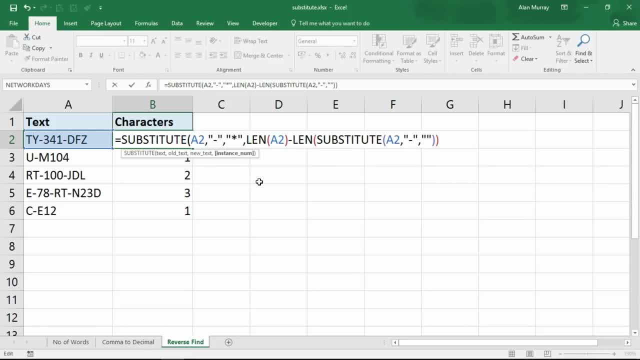 I have made the most of that. But that is a real special part Of the substitute function That really differentiates it From some of the other text functions available: That you are prompted For an instance of that character, Like what instance of the hyphen? 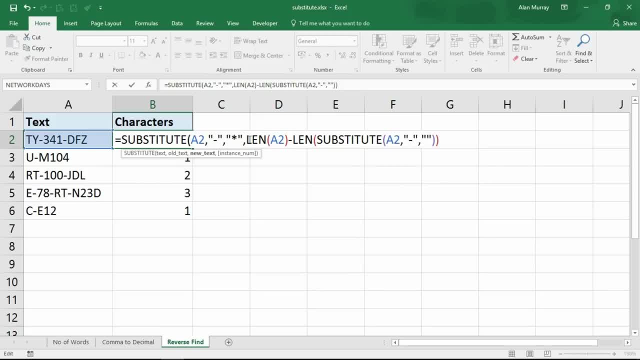 Are you interested in? Is there a specific one? Well, yes, there is The last one. I want to put a flag in the last one, The final occurrence. The formula we had beforehand Is how many hyphens there are: AKA. 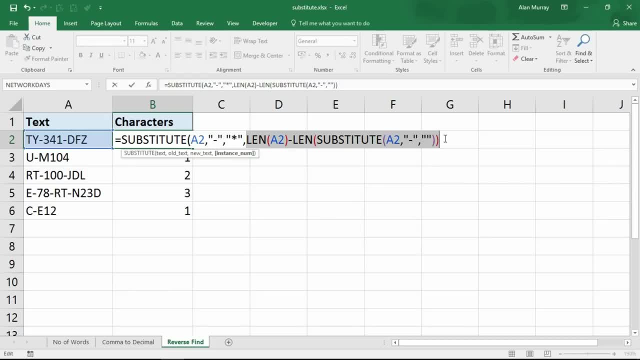 The position of the last one. So if I just click on the end And put a closed bracket And press enter, The point we are at now Is that we have put down a flag, Put down a marker In the final occurrence. 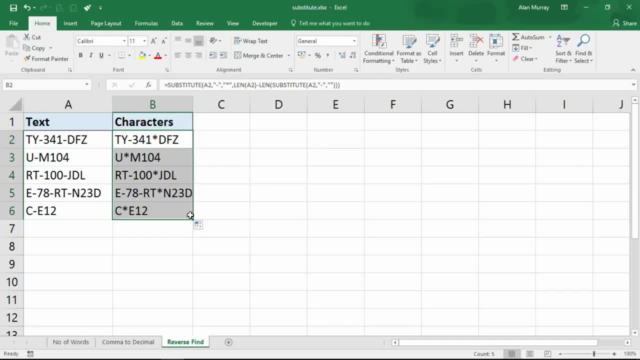 Of a hyphen In each of those cells. Now the final moment Is to get the key Of the characters After that marker. So Last bit here, And this is coming from the write function. Extracting text from the. 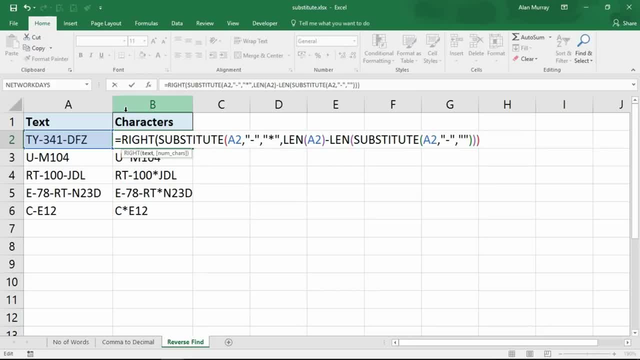 Like characters from the end of a cell Write function Wants to know where the text is. It's A2.. Comma: How many characters? Well, that's the difficult question. So I've done once or twice in this video already. 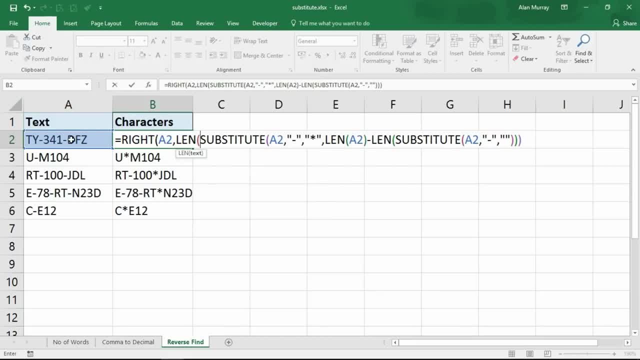 Len functions getting involved, So that I can find out How many characters are there In total And I'm just going to subtract from that The position Of the flag, The position of the asterisk, So I can do that.